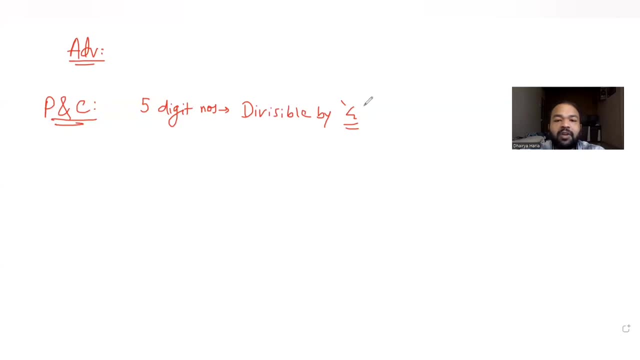 the set of numbers from one to five, which are divisible by four. So the options of choosing the numbers we have. We need to form a five digit number which are divisible by four, And it is also set to us that reputation of digits is allowed, So we have been also. 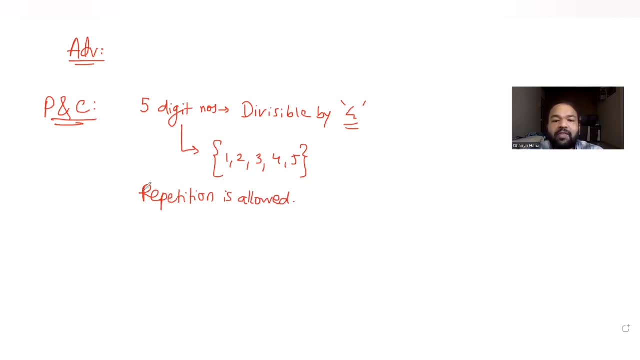 told that reputation is allowed. Let's find out how many five digit numbers we can form here. There are four options given to us: A, B, C, D. A option which is given to us is 3, 1, 2, 5.. B is given 625.. C is given 125.. And the option D is given 165.. So we 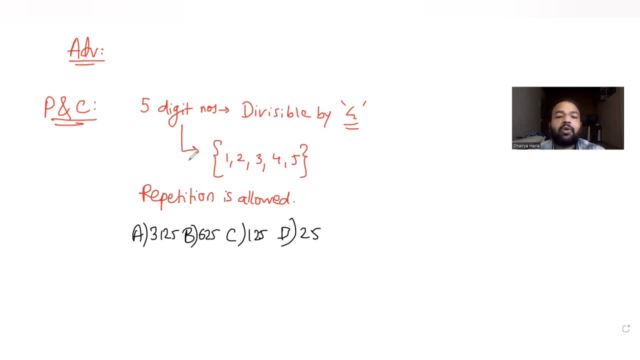 need to form five digit numbers which are divisible by four, And it is also said, to which is there is given process. So we need to figure out how many five digit numbers I can form with this such that it is divisible by four. Let's do that. So if I try to find, 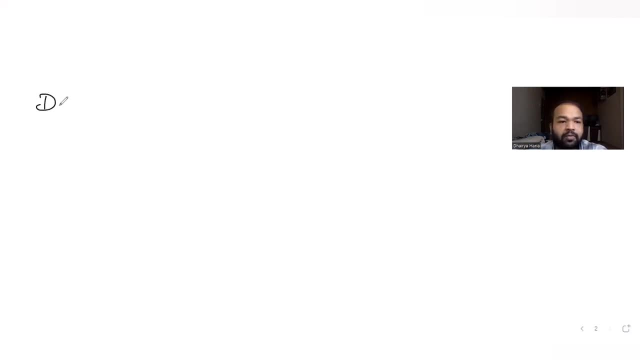 the solution. first thing, if I need to understand, to find if the numbers are divisible by four, if I use the divisibility test of four it says that last two digits if are divisible by four, then I can say the entire number is divisible by four. So I want to form a five. 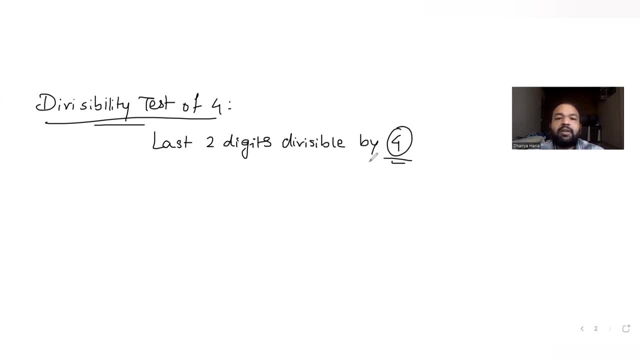 digit number. I just need to check that whether the last two digits are divisible by four or not. Example: if I show it to you. let's say, if I have a five digit number, I just need to check that whether the last two digits are divisible by four. that is 32. 32 is divisible by four because 32 by 4 gives you 8. 4 8s are 32. so 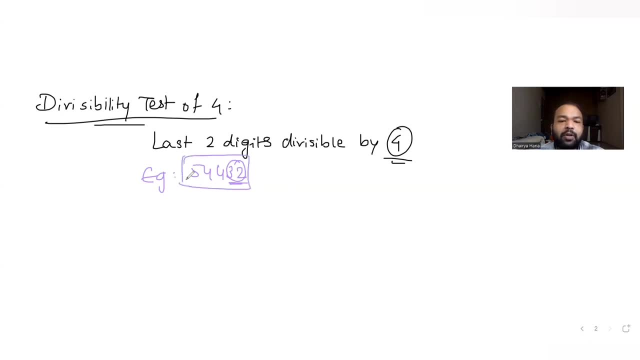 32 is divisible by 4, I can say that entire number, five digit number, is also divisible by 4.. So the idea is we are just going to understand the last two digits and we'll check for how many numbers the last two digits are divisible by four. So let's understand that. 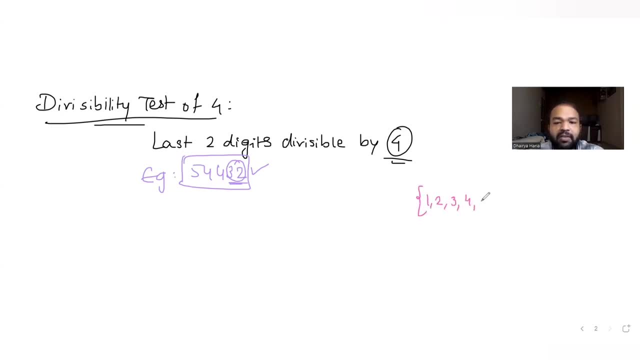 the options of numbers to be selected from 1 to 5. if i take two digits at a time, i can have 1, 2, 1, 3, 1, 4, 1, 5. i can have with 2 as the first digit. i can have 2- 1. i can also have 1- 1 here because 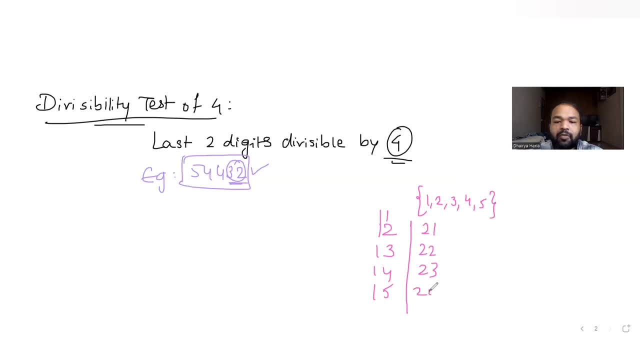 reputation is allowed: 2 1, 2, 2, 2, 3, 2, 4, 2, 5. i can have 3 1, 3, 2, 3, 3, 3, 4, 3, 5. i can have 4 1. 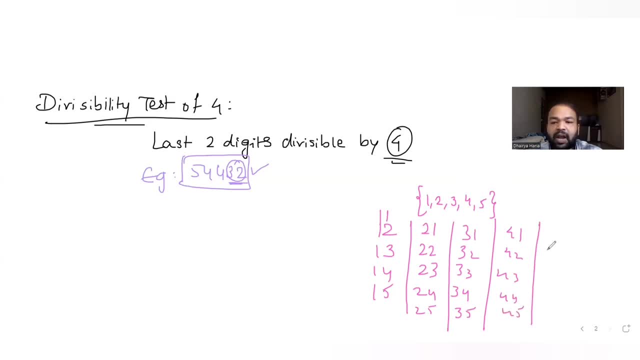 4, 2, 4, 3, and the last option i can have is 5 and 5, so 20 options of two digit numbers i can form with this set of five numbers and if i see here, 12 is divisible by 4 out of these five numbers. 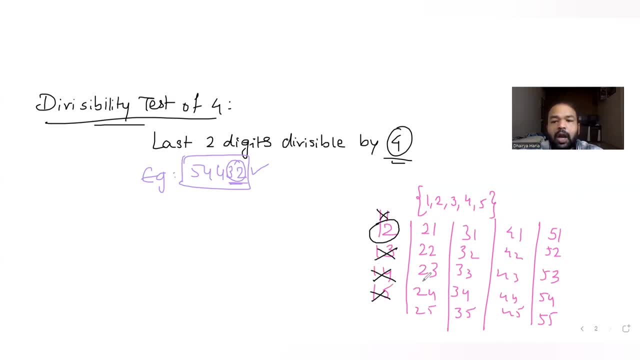 the others are not divisible by 4. out of this set of five numbers, again 24 is divisible. the other four numbers are not divisible. out of this set of five numbers, again 32 is divisible. the other four are not. out of this set, i know 44 is divisible, others are not. 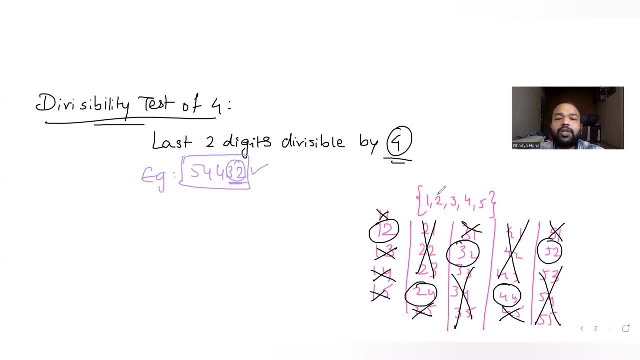 so i understand, out of the total list of two digit numbers which i can have at the end, i understand there are four numbers or five numbers which are divisible here. that is, 12, 52, 54. so we have this, so we have these five numbers at the end, which tells us that they are divisible by four. 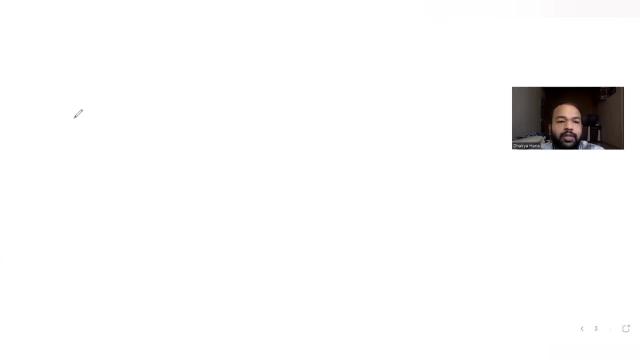 so now i have this five options to select from for the last two digits. so if i make the arrangement here- five digit numbers, i have to arrange them and out of five digits. i have been told that this last two digits has five options, so i need to select any one out of those five so that can be. 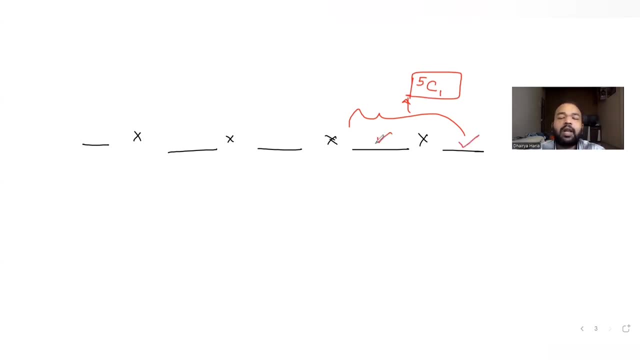 done in five c one ways, which will help us to select last two digits and for the first three digits i can have any one of the five numbers, because it's told to me that the repetition of the digits is allowed. since the repetition is allowed, i can. 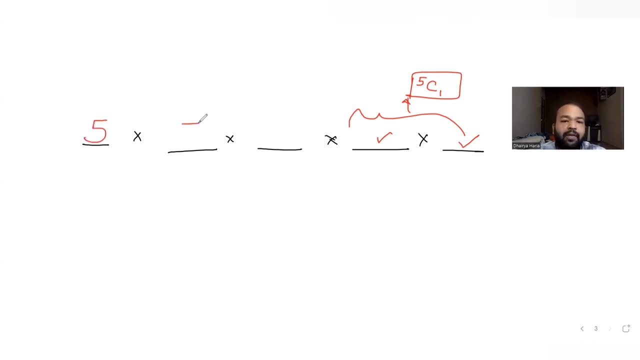 have any one out of five numbers? with whose position? any one out of five numbers for the second position as well, and any one out of five numbers, for this gives us number of five digit numbers divisible by so if i find out how many phone digit five digit numbers are there, which?